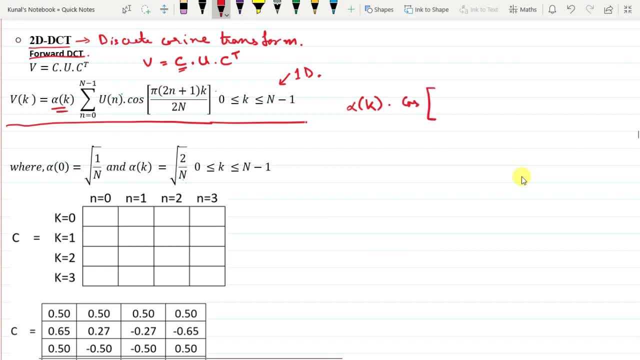 by cos of Pi into 2N plus 1 into K divided by 2N. Now for a 2 by 2 DCT matrix. our high density matrix must be 0 and��baly accepted. Now we are going to talk about the quieresilities of Deposit and Answer. 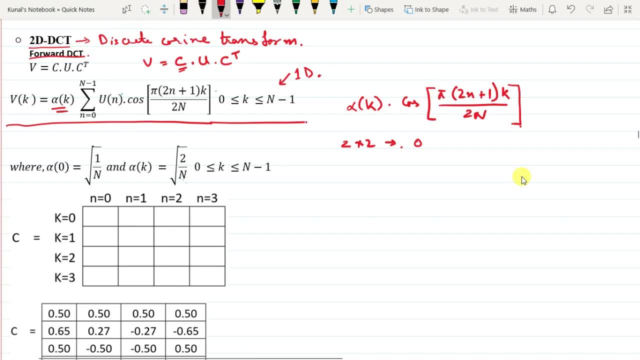 our n and our k values. n comma, k values: it varies from 0 to 1.. Okay, So for the calculation of this we will be making a 2 by 2 matrix and over here we will be varying. say n equals. 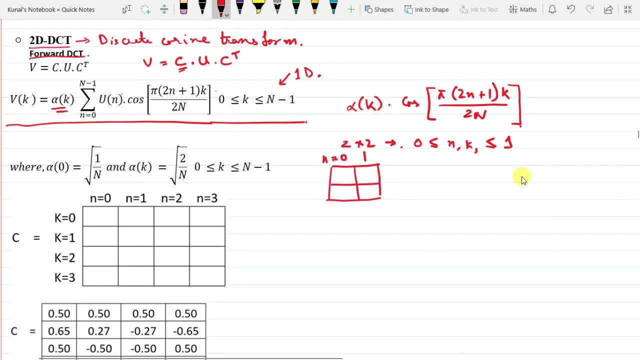 to 0, 1, and in the y axis it will be: k equals to 0 and 1.. Further, in any case, alpha 0 is equal to under root of 1 by n. In this case, capital N is equal to 2.. So it will. 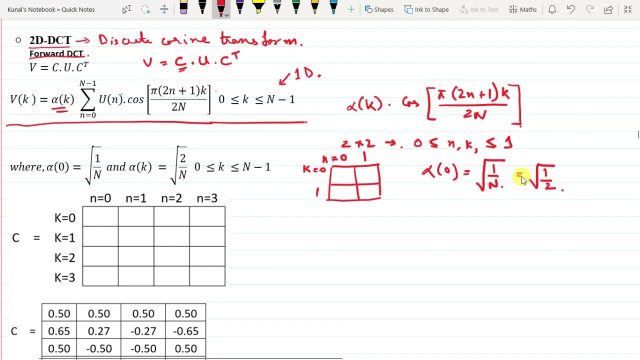 be under root of 1 by 2.. Now what happens over here is that, for, k equals to 0, that means all the values in this rows will be having a value of under root of 1 by 2.. Okay, So let us write it. 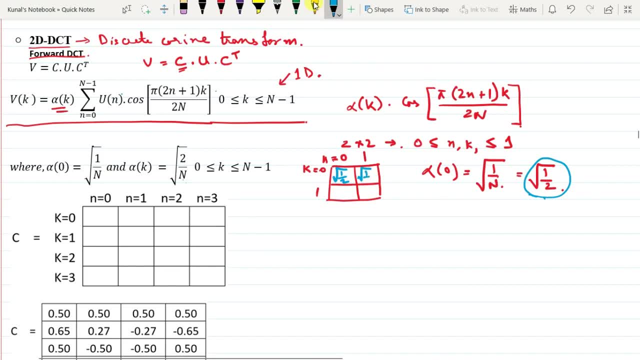 down under root of 1 by 2 and under root of 1 by 2.. Right Next. So we will cancel. our n is equal to 0 and our k is equal to 1.. So our alpha k, it will. 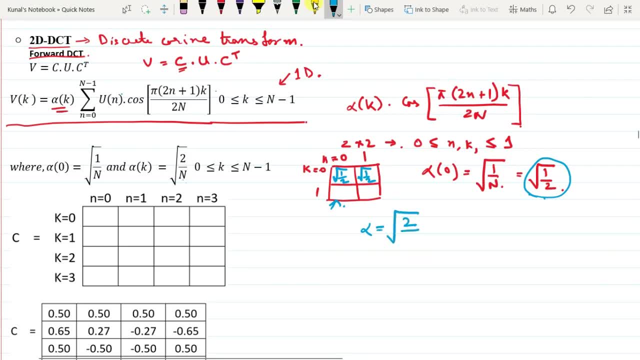 be under root of 2 by n, again 2.. So this gets cancelled out, So this becomes 1.. So right, Then our this portion. it becomes cos of pi 2n. So 2 multiplied by 0 is 0 plus 1. So. 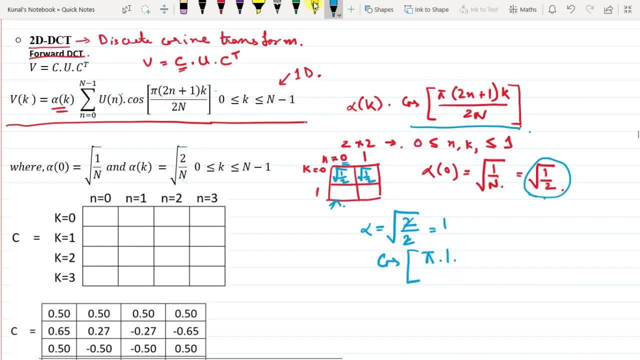 it becomes, multiplied by 1, multiplied by again, k is equal to 1, divided by 2 into 2, 4.. So it becomes cos of pi by 4.. Right, So our alpha k was 1 and this is again cos of 4.. So cos pi by 4.. So this box, it assumes. 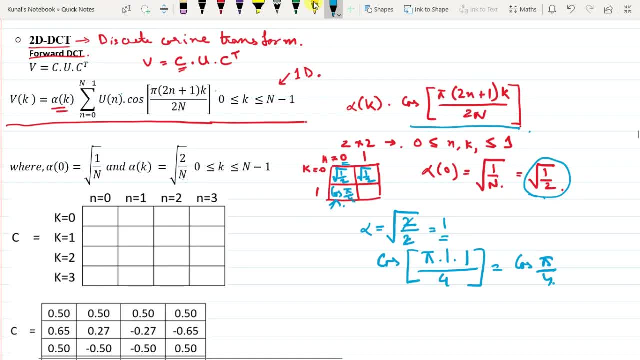 the value of cos of pi by 4.. Similarly, when we go to this last pixel, where n is equal to 1 and k is equal to 1. Again this alpha value, k equals to 1. So it becomes 2 by n. 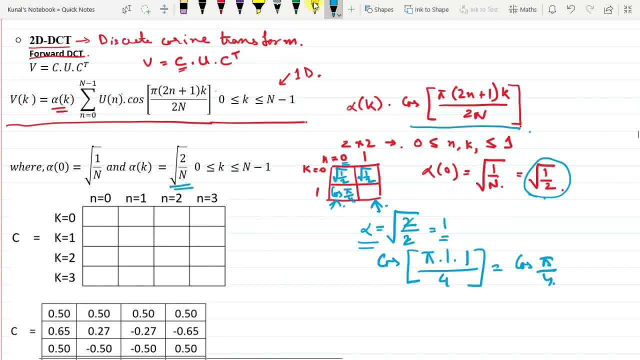 Right. So this becomes 2 by under root of n. That means 1 again, and then this value: it becomes cos of pi into 2, into 1 plus 1, 3 multiplied by 1 by 4.. So it becomes cos of 3 pi by 4.. 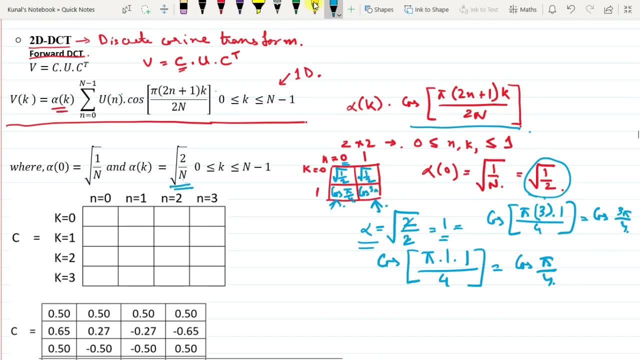 So this assumes the values of cos of 3 pi by 4.. So you can calculate the values over here. Similarly, when we come, when we are deriving the 4 by 4 matrix, our 4 by 4 matrix, it assumes this value. Over here we are having n equals. 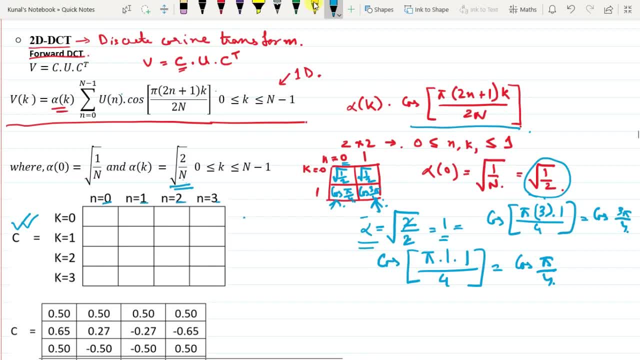 to n varies from 0,, 1,, 2,, 3, and k varies from 0,, 1,, 2,, 3. again Now, when k equals to 0, this our alpha 0, it will become 0. 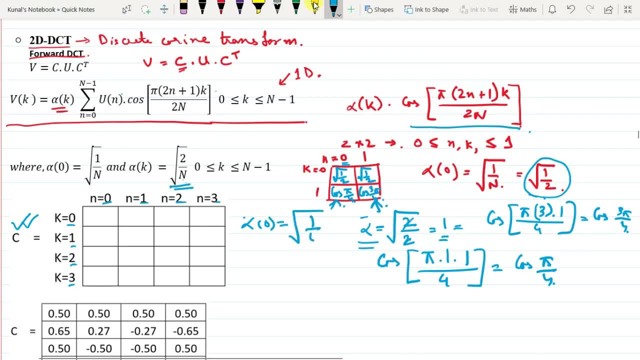 Right, So we get 1 by 4,, which is equals to 1 by 2.. Okay, And in all these cases, since k equals to 0,, we will get cos of 0,, which is equal to 1.. So, multiplied by this one, So we get: 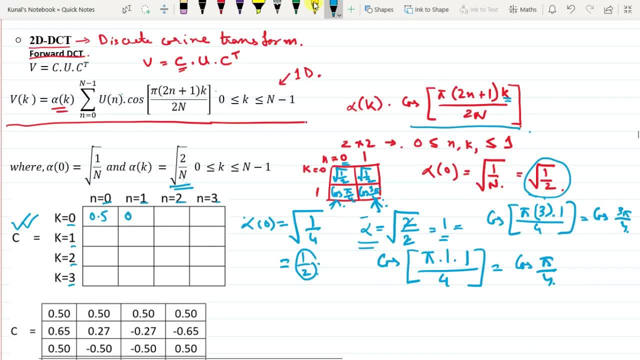 multiplied by half, So we get 0.5 in all the pixel values. Okay, Okay, Okay Okay. Then for the calculation of the other pixels we will use alpha. k equals to under root of 2 by 4, which is equals to under root of 1 by 2.. So for k equals to 1, all these values 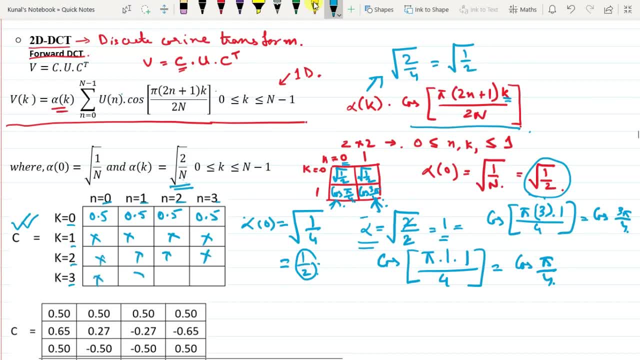 then k equals to 2, all these pixel values or these matrix values we will consider alpha. k equals to under root of 1 by 2.. And we will change the values of n and k in this cos function and subsequently we will get the values. So I have already calculated the value over here. 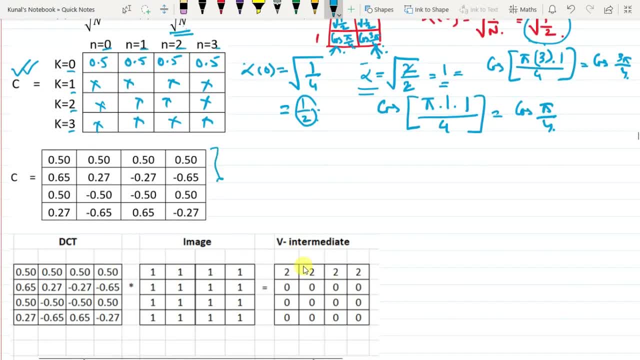 and this is the matrix which we have got Now for the calculation of the DCT image. Now what we have to do is that, as I already said you that we have to multiply, for calculating this DCT domain image, or DCT transformed image V, we have to multiply c multiplied by our 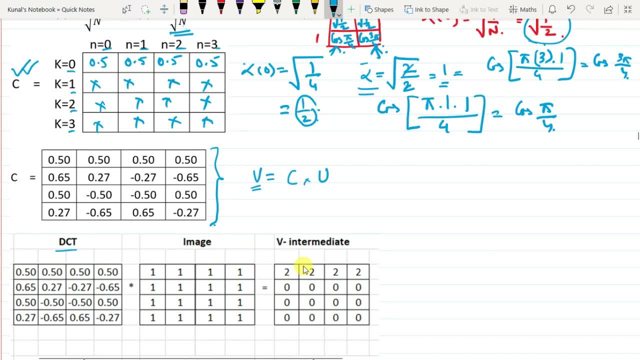 image u. So this is what I have done in the first step: DCT multiplied by image and we have got the intermediate image. Okay, Okay. So then I will multiply this V intermediate with transpose of the c matrix, which is the. 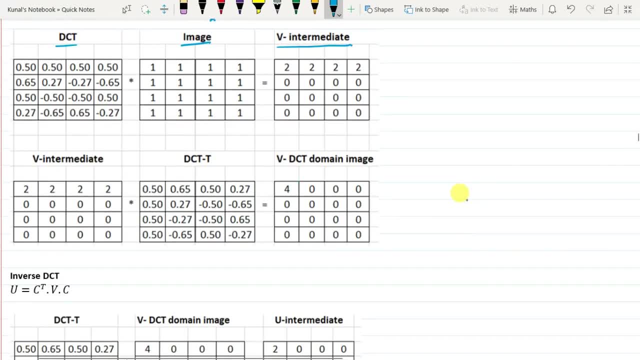 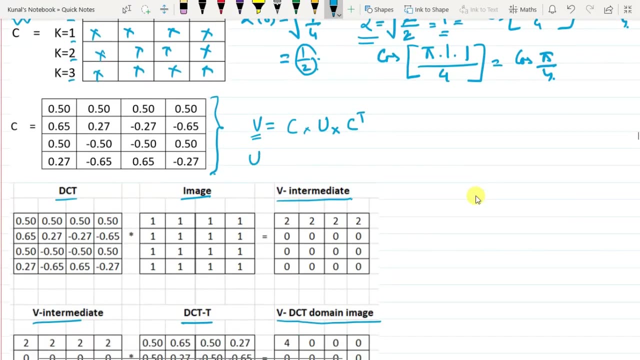 DCT transformed matrix. So again over here. So we will be getting the DCT domain image Again for the calculation of u. that is, to get back the original image. Take from the transformed image. We will be going for a reverse transformation process. 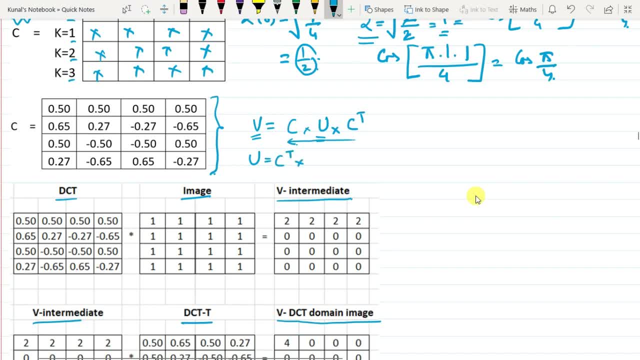 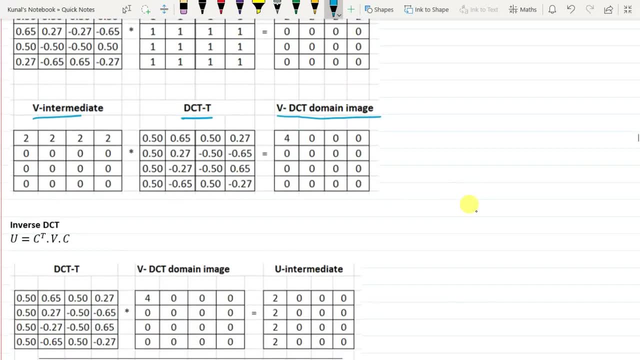 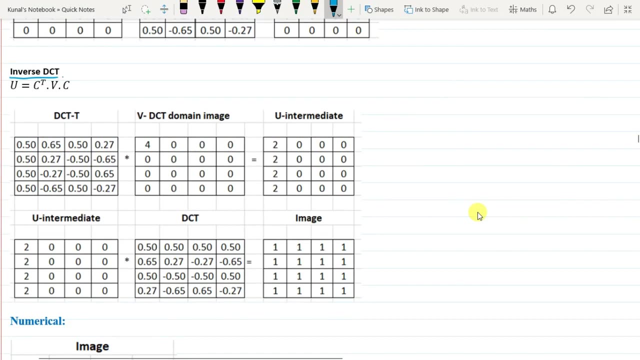 that mean that we will be multiplying ct with V and again then with c. Okay, so this is what I have done over here for calculating the inverse DCT. So u equals to ct multiplied by V, multiplied by c, and I have calculated all these values. 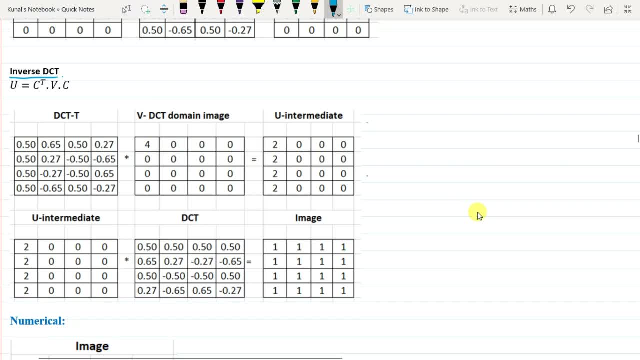 and consequently, If you see, after doing so, first I have multiplied with this DCT transpose with the transformed image and I have got U intermediate, and then again with the U intermediate, when I multiplied with the DCT matrix, I got the original image. Okay, so this is how we can calculate the DCT matrix and how we can get into the DCT transformed image and again back from the transformed image to the original spatial domain image. 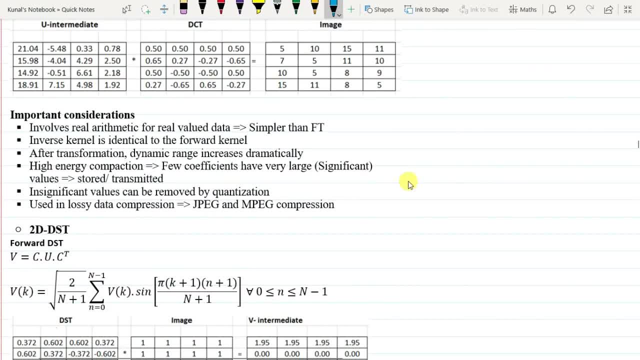 Now there are certain considerations over here which you would be needing if I give some numeric. I give some of this short note on DCT. first of all, it involves DCT involves real arithmetic for real valued data and because of this reason it is simpler than FT, where FT has got conjugate numbers and we have to deal with the sorry complex numbers not conjugate. 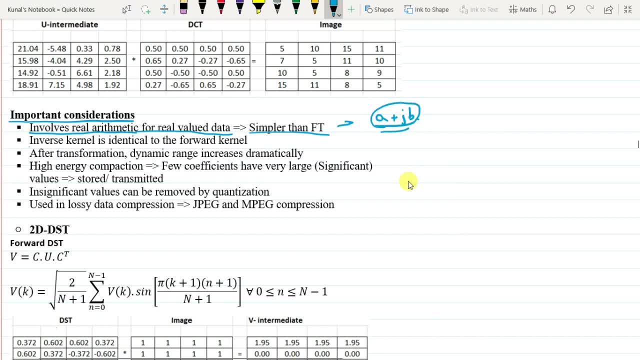 It is having the complex numbers and we have to deal with the complex multiplication and addition. Again over here, inverse kernel is identical to the forward kernel. this is another important thing. in the case of Fourier transform, we had to take the conjugate. okay. so forward transform and the inverse transform, they were different. 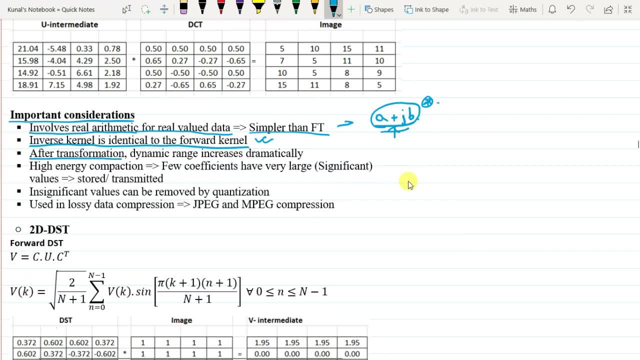 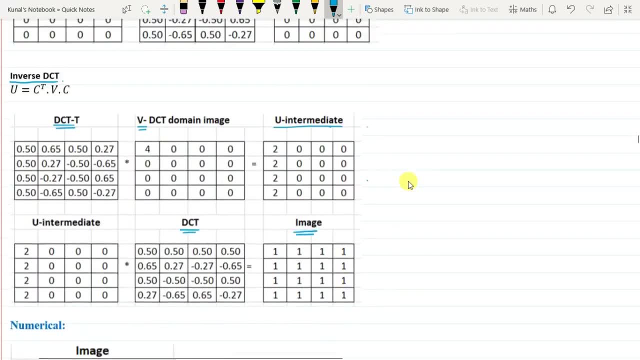 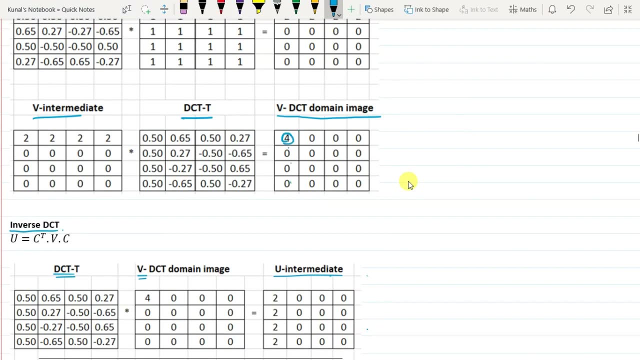 Then after transformation, dynamic range increases dynamically. okay, if you look into here into the DCT domain image, Frog has the favorite animated box- we have got four over here and all other values are zero. So if you look into the image, it is a highly correlated image and DCT helps us in data compression. we get only one- significant numbers- and the rest are insignificant numbers. 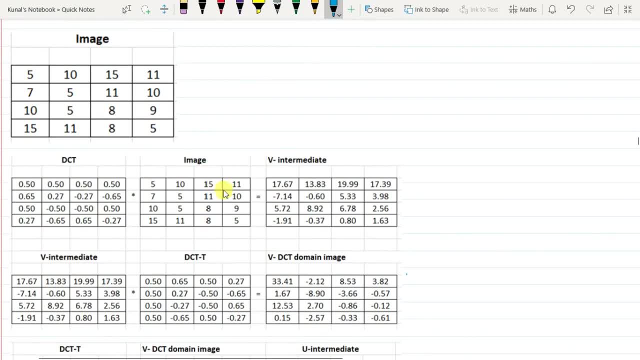 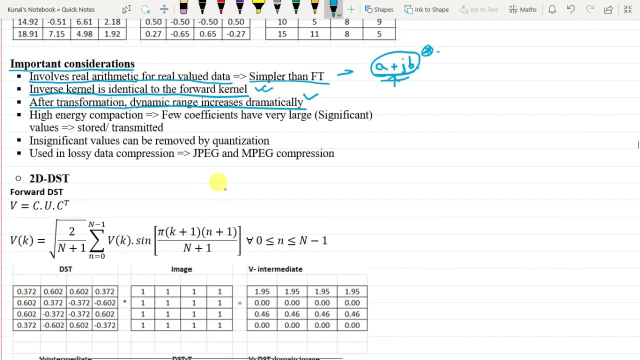 Again in another example. if you see, in this image we have got this significant number and the first number should be 0. pixel, 00 pixel and all other pixel values are not that significant. So because of this there is a dynamic increase in the dynamic range increases dramatically. 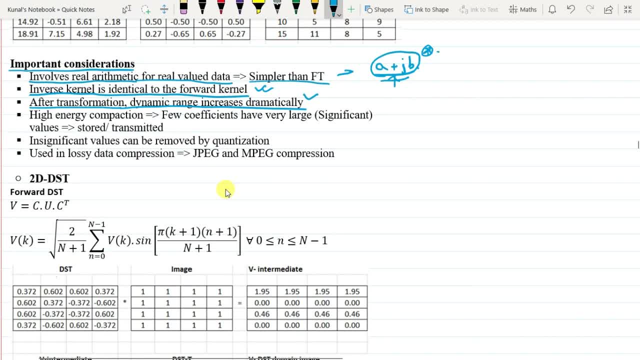 and then because of the reason already I have told, that only one pixel, 00 pixel, has got the significant digit and all other pixel values assumes very negligible value. So this helps us in high energy compaction. This is because few coefficients have large or significant values.